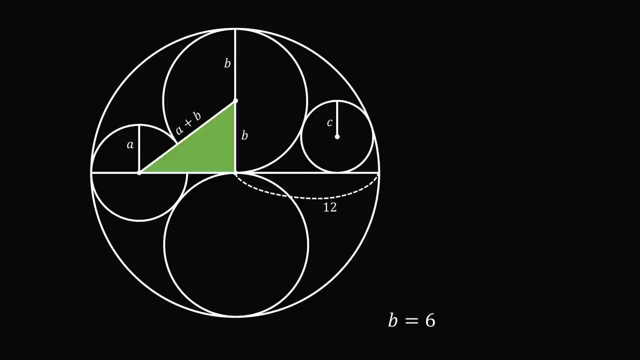 What's the length of the other leg of this right triangle? We know that this length is equal to a and a radius of the large circle is equal to 12, so the other leg will have length equal to 12 minus a. Since we have a right triangle, we have the square of a plus b. 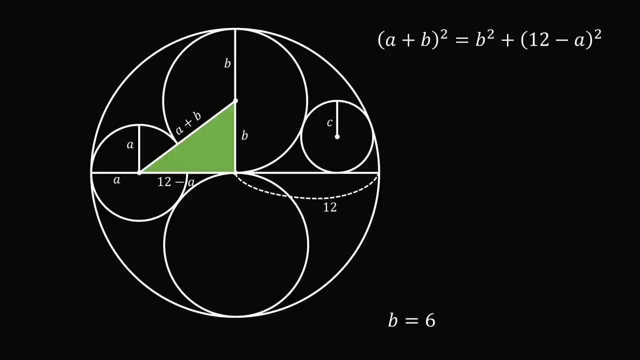 is equal to b squared plus the square of 12 minus a, Substituting in that b is equal to 6, we can simplify this equation and we can work out that a is going to be equal to 4.. So now let's work out the value of c. 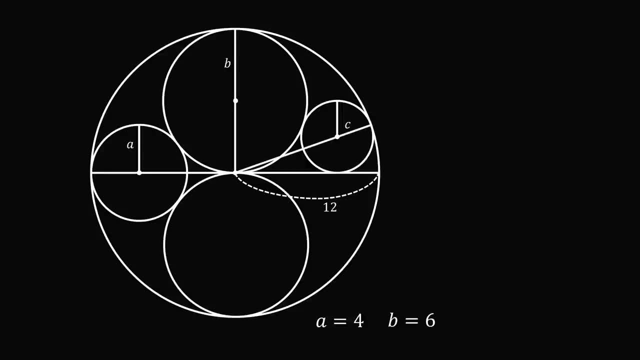 We will first construct the following radius of the large circle. This will have length equal to 12.. Next, construct this radius, which has length equal to c. Now we have a right triangle here where one leg is equal to c. The length of the hypotenuse will be the length of the radius of the large circle. 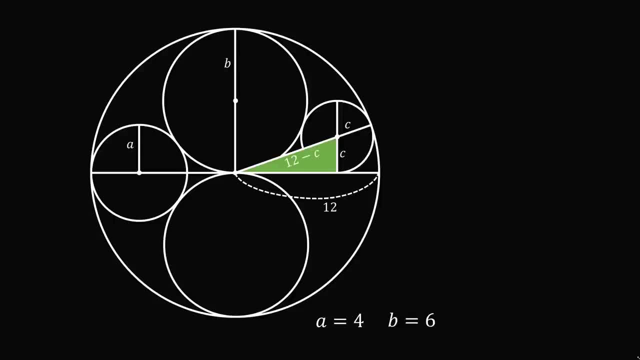 minus the length of the radius of the small circle, so its length will be equal to 12 minus c. Let the length of the other leg be equal to x. Now let's solve for x squared. Since we have a right triangle, x squared is equal to the square of 12 minus a. 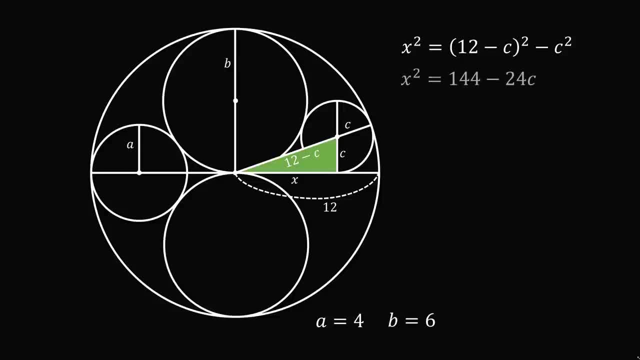 We can simplify this equation to get x squared is equal to 144 minus 24c. Now let's construct the following right triangle: One leg will be equal to x. The other leg will be the difference in the length of the radii, so it will be equal to b minus c. 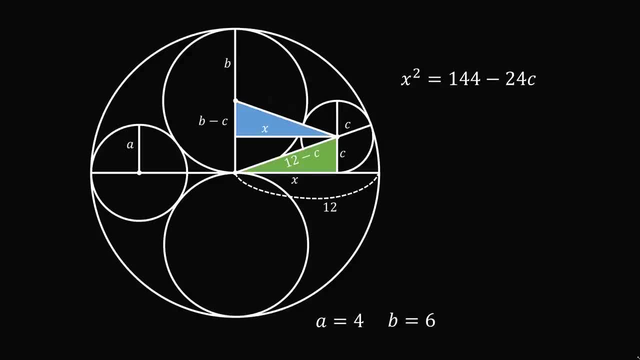 The hypotenuse will be the sum of the radii lengths, so it will be equal to b plus c. Now let's solve for x squared. in this right triangle We have, x squared is equal to the square of b plus c, minus the square of b minus c. 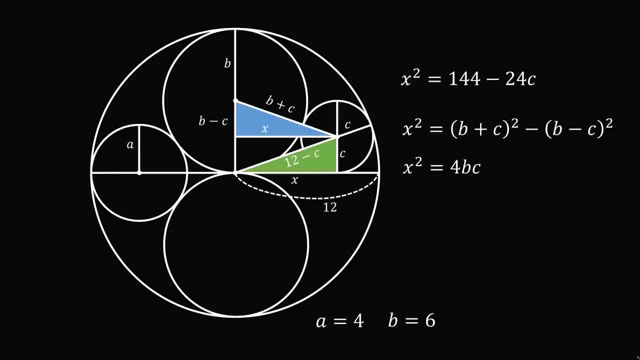 We can simplify this equation to get x, squared is equal to 4bc. Now we can substitute in that b is equal to 6.. So we have x, squared is equal to 24c. So we can now focus on these two equations and we can set them equal to each other. 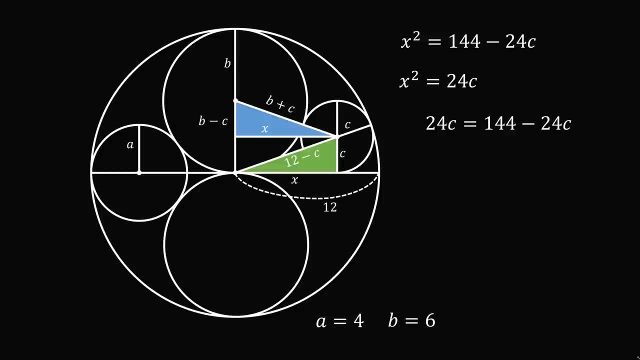 So we have: 24c is equal to 144 minus 24c. Simplifying we'll give that c is equal to 3.. So we've solved for the values of a, b and c And this gives that a plus b plus c is equal to 4 plus 6 plus 3..